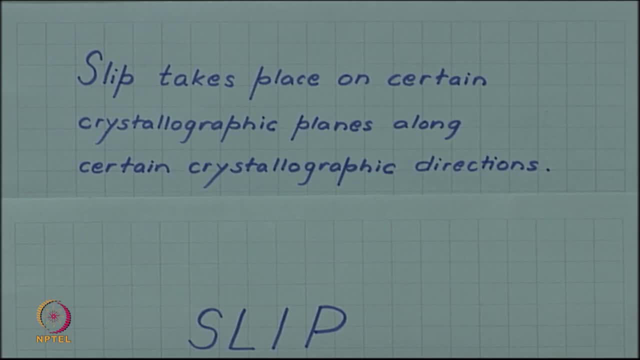 planes along certain crystallographic directions. So when slip became important in the consciousness of scientists working on plastic deformation, they started doing careful experiments. and these require lot of careful experiment on single crystals and with X-ray diffraction, because you have to find the orientations of the crystal before deformation and after. 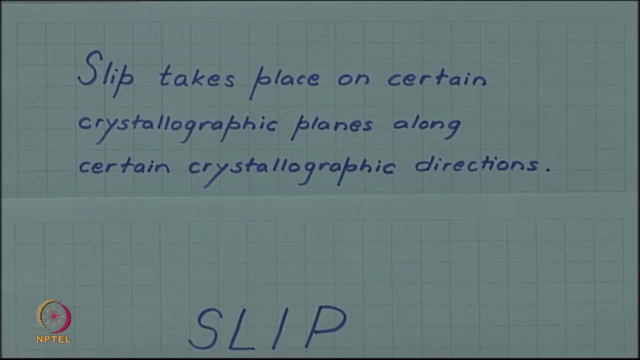 deformation. So such careful experiments then established that slip is taking place in any given material, in any given crystal when you are deforming. Slip takes place on certain crystallographic planes, along certain crystallographic directions. By crystallographic I mean that certain, a particular specific Miller indices of the plane, particular orientation. 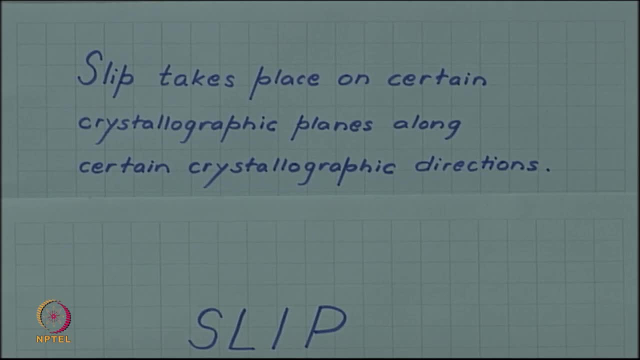 of the plane will be suitable for slip, not all planes, and similarly, certain crystallographic directions will be suitable for slip and not any arbitrary direction. Then the next interesting thing was that these slip planes, which they found the crystallographic planes for slip, they were known as slip planes and the crystallographic directions were the 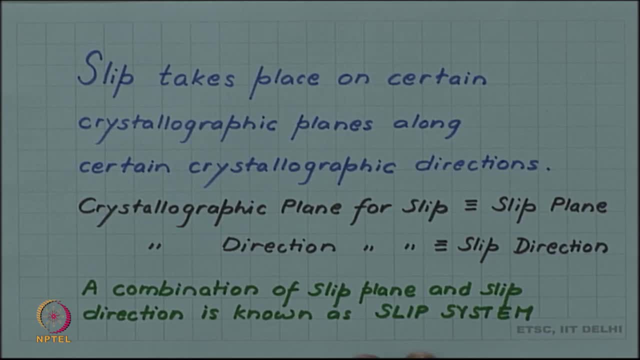 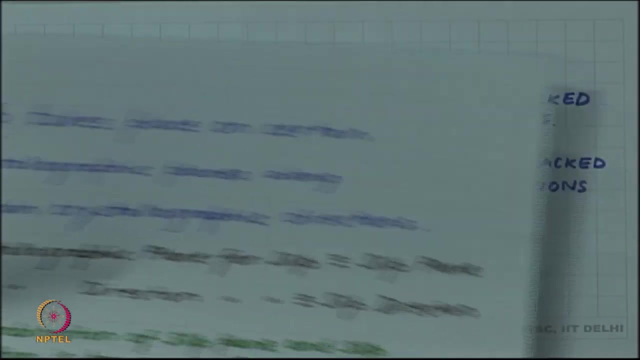 slip direction. We also have a term called slip system, which is a combination of slip plane and slip direction lying in that plane. So with this terminology- slip plane, slip direction and slip system- Let us look at the next example. 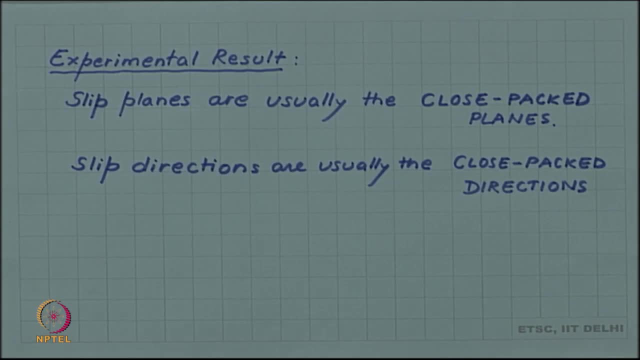 The next interesting result, and again an experimental result, that slip planes are usually the close packed planes. So we have seen various crystal structures and we have seen that particularly in cubic close packed and hexagonal close packed crystals, there are certain planes which are very high density of packing and they are the close packed planes. 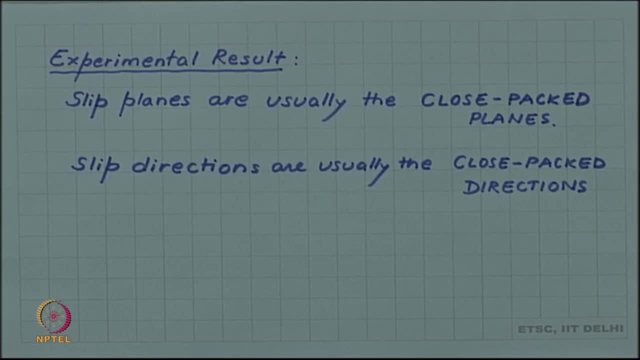 And similarly certain directions are close packed directions. For example, in cubic close packed structure the phase diagonals are the close packed directions, So slip was happening. when these experiments were performed they found that the slip was happening on these closed packed plane, in these closed packed directions of course. So this again through. 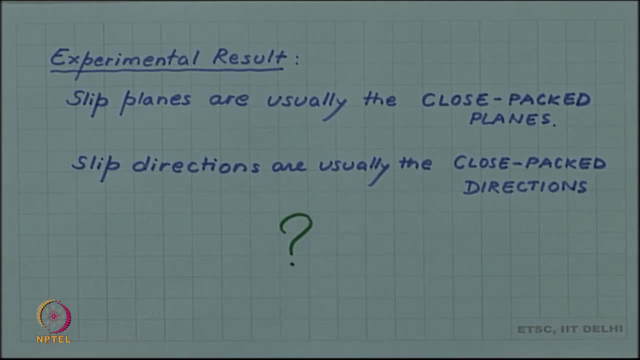 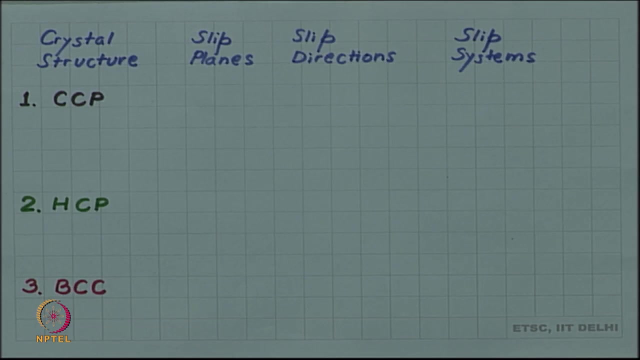 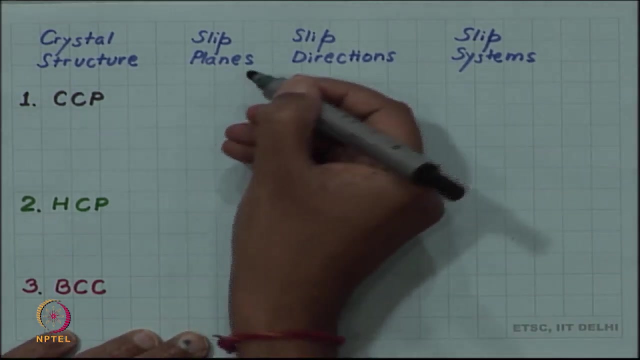 a question that why closed packed plane and closed packed directions are being favoured. We will look at it as we go along, but let us first note down what result they found for different crystal structures. So for cubic, close packed structure, as you know, CCP, the slip planes, if you want the close packed planes, the close packed planes. 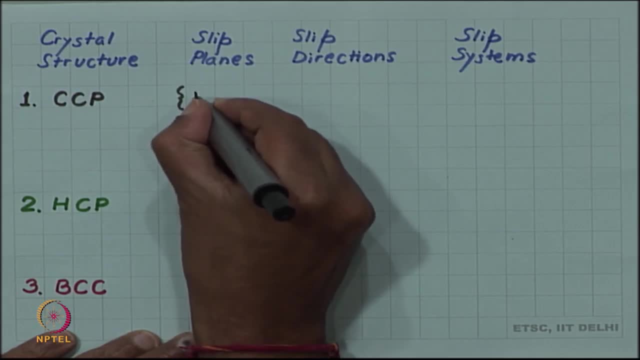 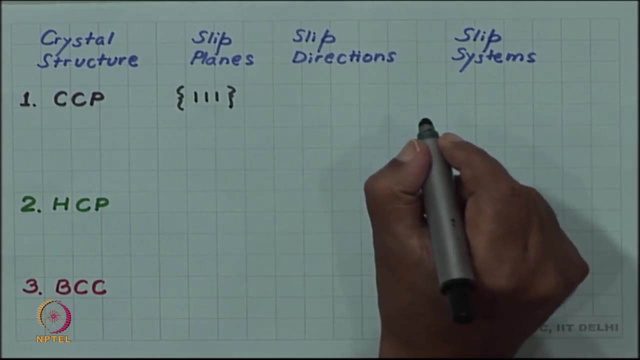 in the cubic close packed structure are of the 1 1- 1 type. You will need to review some of your crystallography videos which we have seen. we have discussed these things So close packed planes in CCP are of the 1 1- 1 type and the slip direction if it is a close. 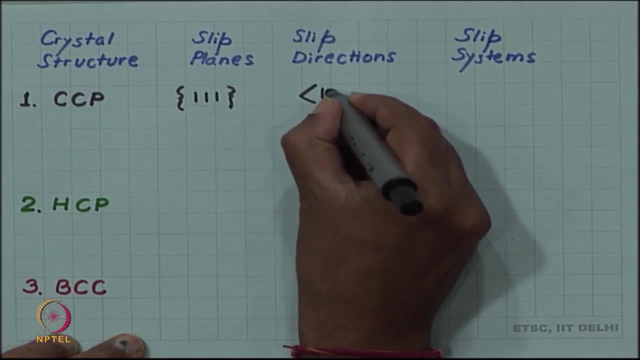 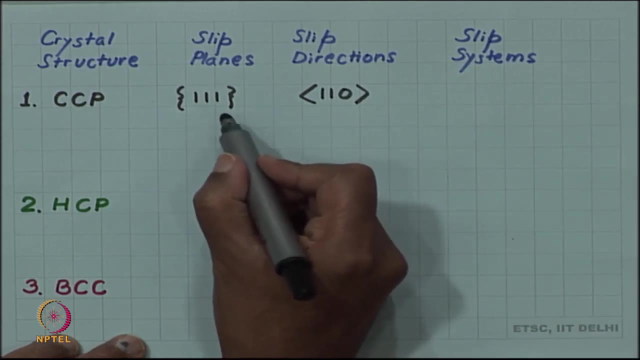 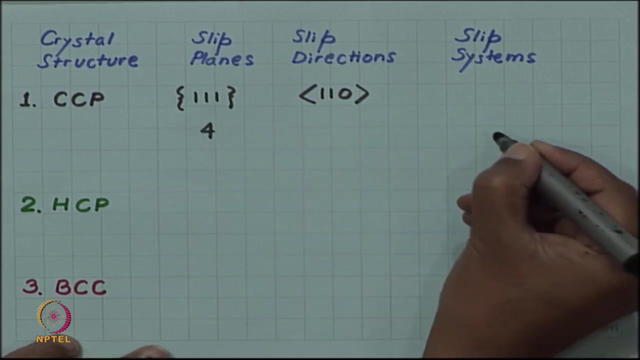 packed direction. So that is of 1: 1, 0 type. what is the use of brackets? I am using curly bracket because it is not 1 1, 1, 1 plane. There are four such planes in the crystal and similarly there are not just one. 1, 1, 1 o j direction. this is a slip direction. 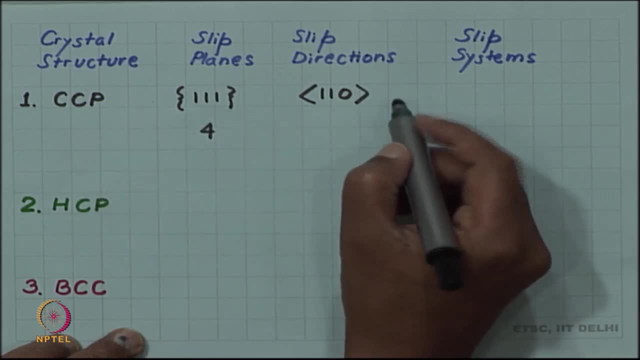 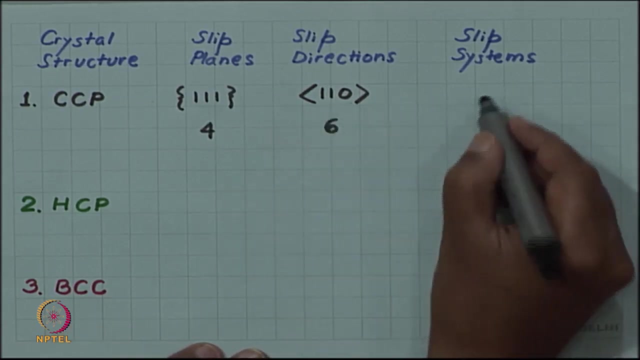 direction. this is a close packed direction in the cubic close packed structure and this is the phase diagonal and there are 6 different phase diagonals in a C C P crystal. So the number here is 6, the total number of slip systems and the way to write the slip. 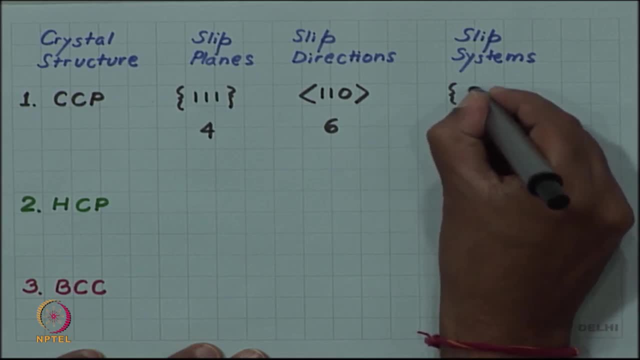 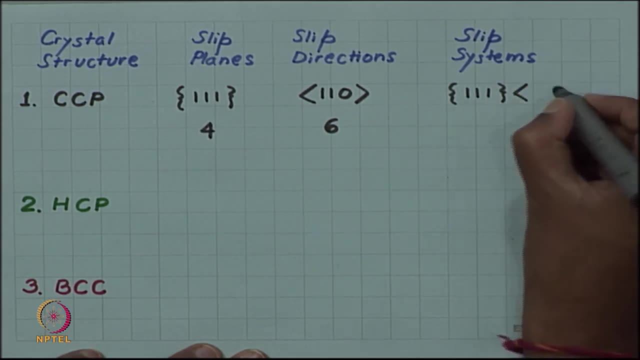 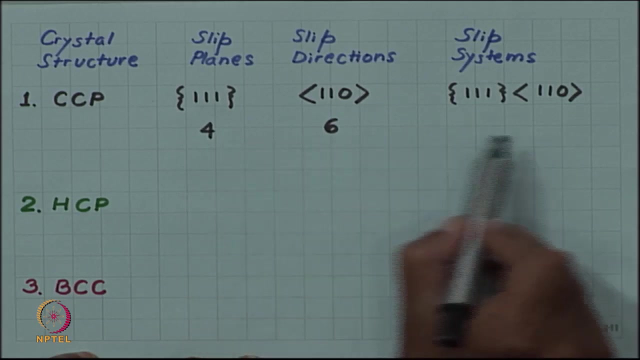 system is to write the plane and direction next to each other. So we will write 1 1 1 and 1 1 O, but recall that. so we have 6 directions and 4 planes. So we may think that there will be 24 slip systems, but not really, because out of these 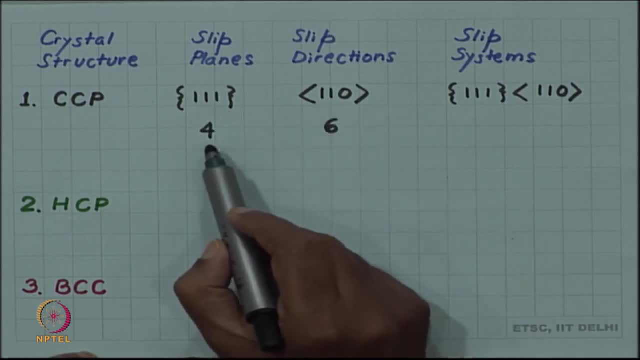 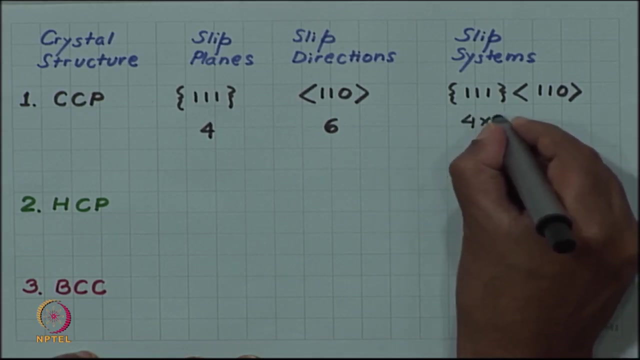 6 directions. all 6 does not lie on each of these 4 planes. So in any given plane only 3 of the slip directions lie. so for every plane we have 3 directions. so for 4 plane we have 12 directions. so 4 into 3, 12 slip systems are there. 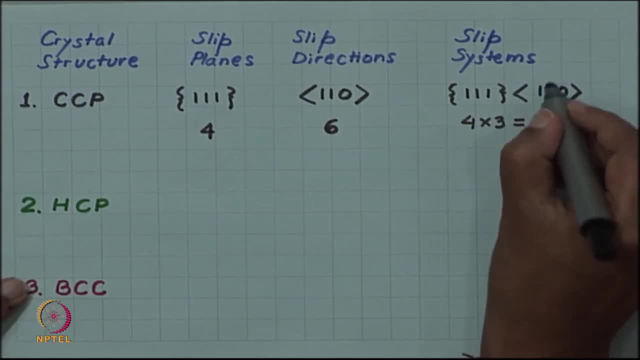 Sometimes, if you really want to be careful, you can insist that the direction lies on the plane so you can satisfy the particular choice which you have made. So you can write for the 3 directions. you will have 7 direction. So in any given plane where the 3 direction lies on the plane I had made using wise Joan. 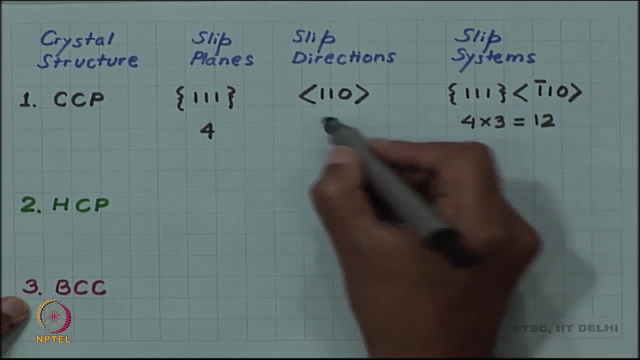 law So I can write bar 1 1 0 instead of 1 1 1, but recall that bar 1 1 0 family is same as 1 1 0 family, because it also belongs to the same family and any member of the family can. 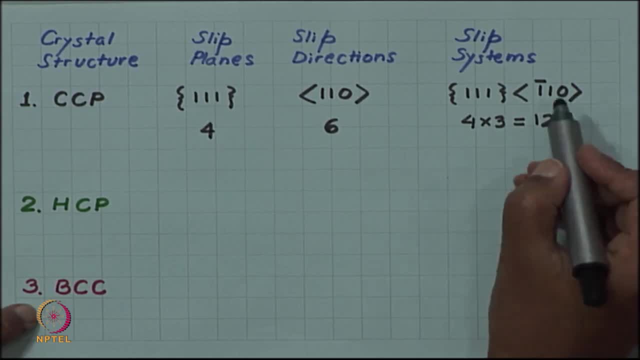 represent the entire family only here. writing as bar 1, 1, 0, then satisfies the wise Joan law with one 1, 1 what I have written here. So it shows that zero Choice is to write 0 와 111 or 2 guilders at the same time, because it is 1 by 2 here. plus and minus, So I can write bar 1 1 0 instead of 1 1 1.. But recall that bar 1 1 0 family is same as 1 1 0 family, because it also belongs to the same family and any member. 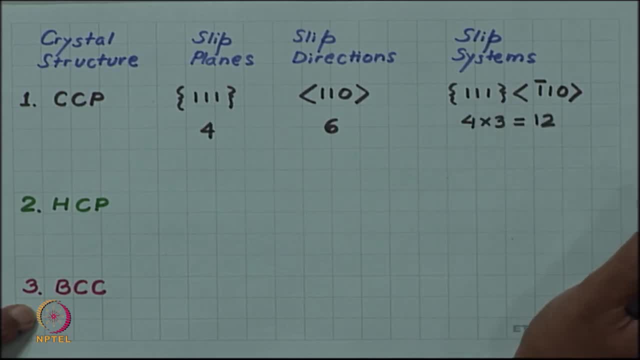 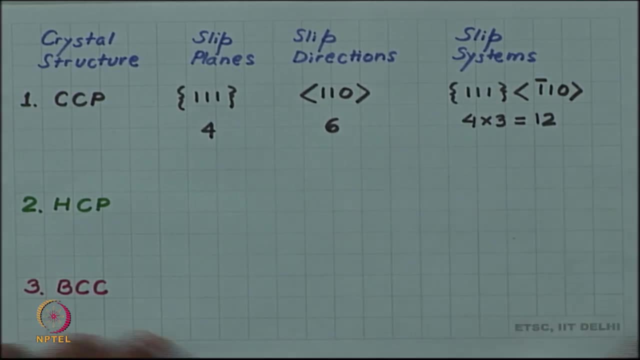 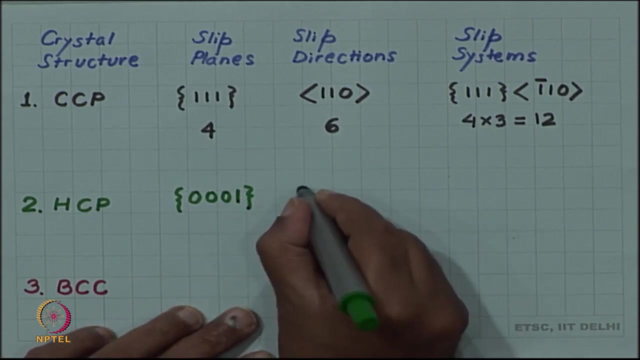 the slip direction should lie on the slip plane and that is why we have 4 into 3, 12 slip systems and not 4 into 6, 24 slip systems. In the hexagonal closed pack system we have the O- O- 1 plane as the slip plane and 1- 2. 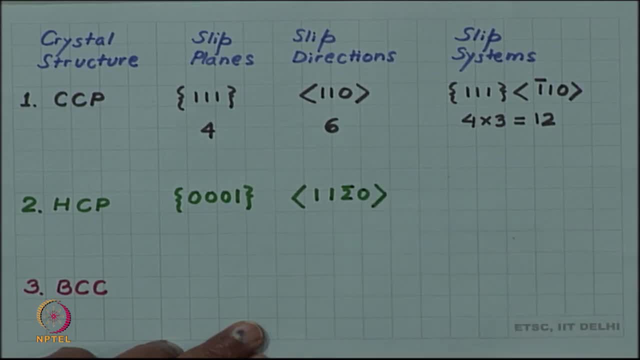 bar. So in the hexagonal closed pack system we have the O, O, 1 plane as the slip plane and 1, 2 bar. So you have 0 direction as the slip direction. So you have this as your slip system. 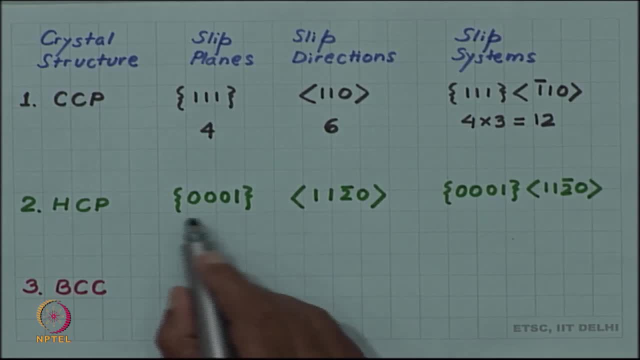 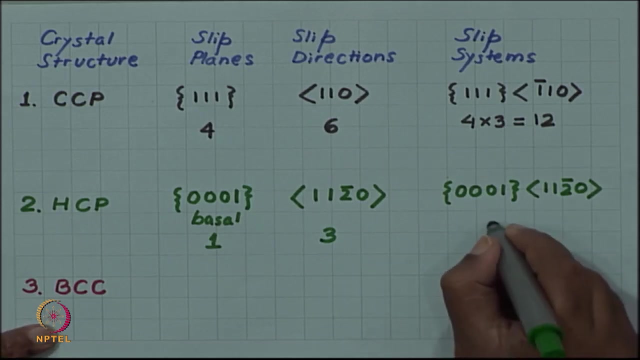 Here, if you think of 0, 0, 1, this is actually a basal plane. This is what is called the basal plane and there is only one set of such plane. and in a given plane, in hexagonal crystal, there are only three such slip directions, three close packed directions. So you have a rather limited 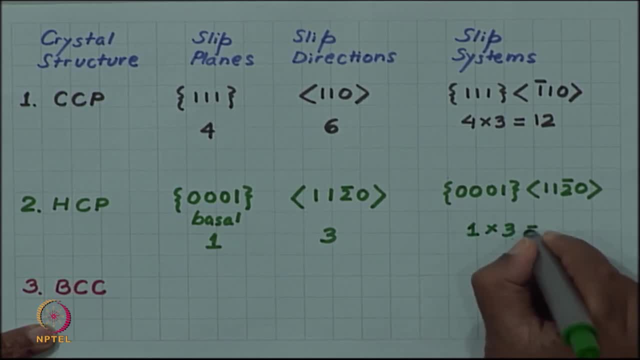 number of slip system. in hexagonal that is only three flip systems. It is an experimental observation that many hexagonal close packed materials are actually brittle, whereas many cubic close packed material are quite ductile, and one reason leading to this sort of behavior is the number of slip system itself. You can see the paucity of 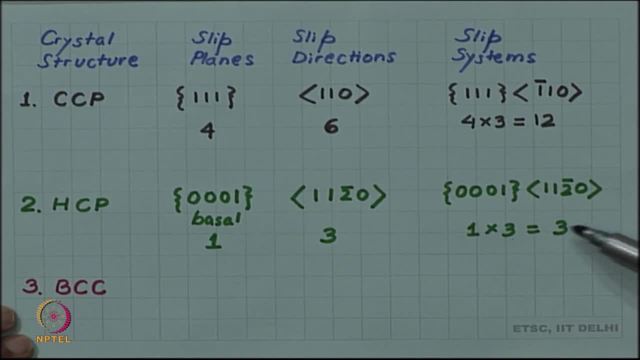 slip system in hexagonal close packed system will lead to a lack of possibility of slipping and that is why lack of possibility of slip And if plastic deformation cannot happen, the material cannot deform and it will behave like a brittle material, whereas cubic, close packed, has a number of slip system and behaves. 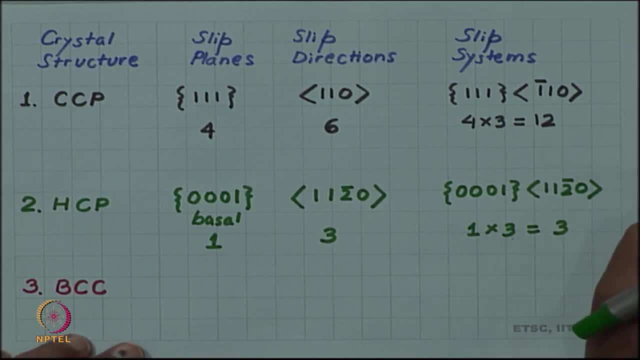 in a ductile manner. This is a very simplistic explanation, but this is one of the pointers towards this made difference in the behavior of CCP and HCP material. Similarly, if you look at BCC, in the BCC there is actually no close packed plane. So 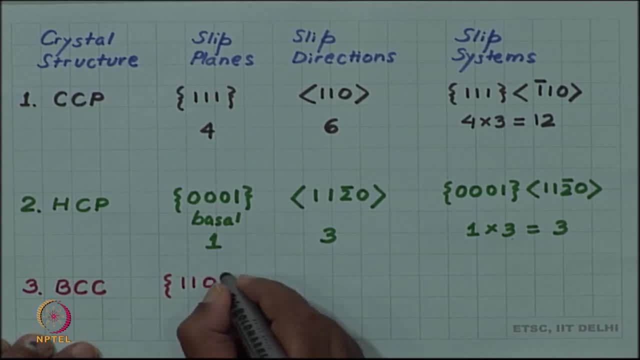 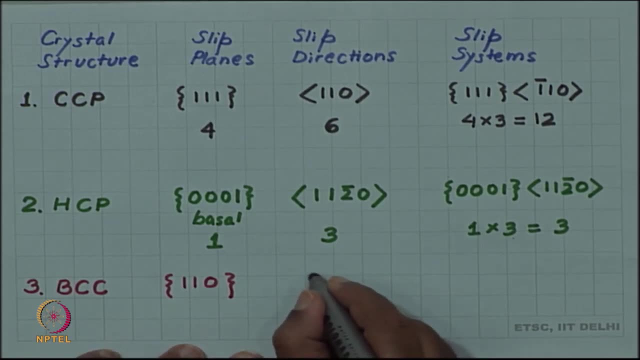 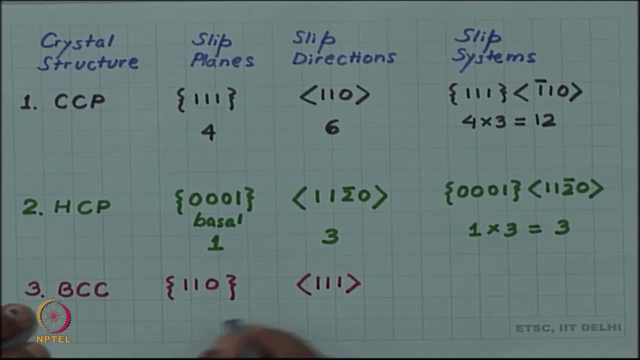 So it is 11.. So it is 11.. So it is 11.. So if you look at the numbers again, this 110 comes out to 6 and this 111 comes out to be 4.. You can see the situation is just reversed from that of CCP. and then you have 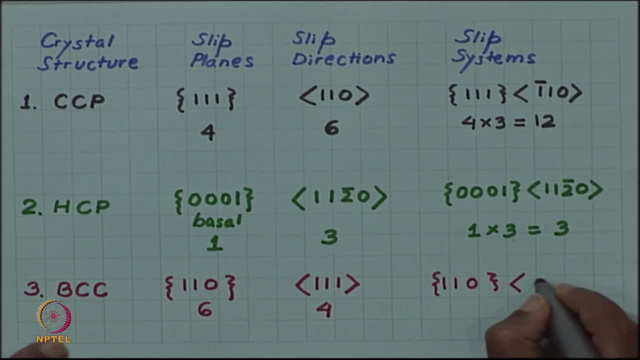 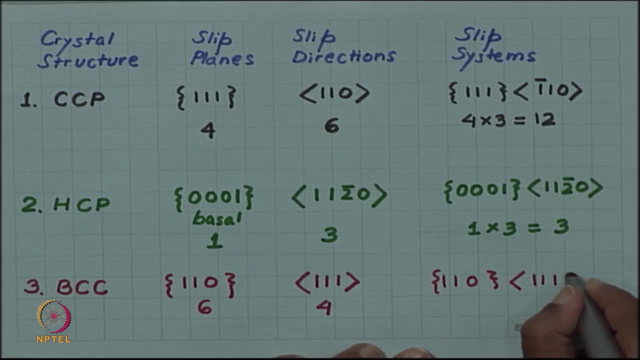 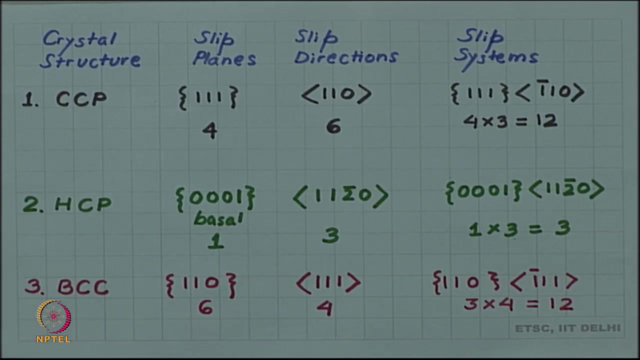 the slip system. So you can do something like this: I can again make it consistent with the Weyers zone law and you will again have 12 slip system. In fact, if I can, so am. I am making a mistake here.